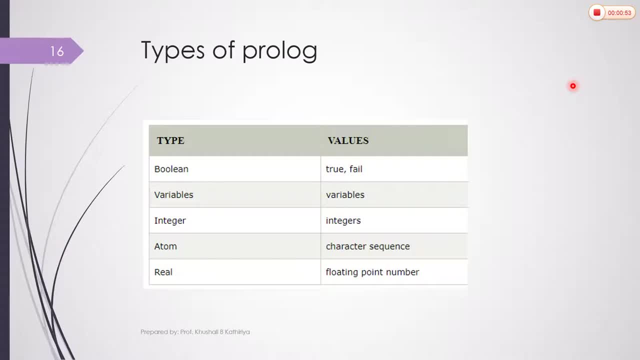 So in this video we will start with the types of prologue. How many types of prologue are available? There are five type of prologues are available. First one is the Boolean. Boolean, that means true and false. You can say binary prologue. Binary prologue, that means zero and one kind of the prologue, Okay. second one is the variables: Variable- that means Boolean, that means either it will be true or false. Okay. so 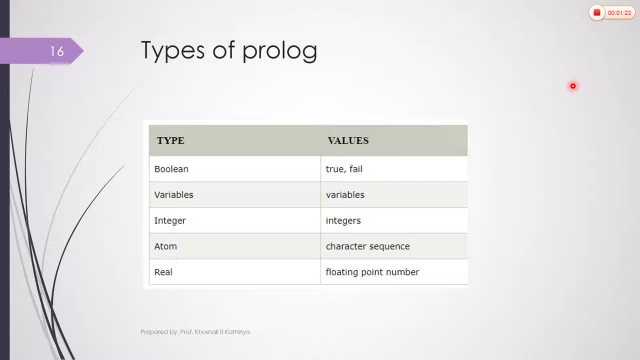 variable. that means prologue are used a variable. Okay, so we can say: second thing as a variable. Third type is the integer. They use the integer integer value, Okay, variable, they used variable. that means a, b, c, x, y, z, like that. If we are using any fact, suppose animal x implies dog x, Okay, so what was the x there? It was a variable. Okay, what was that? It was a variable. Now we have an integer type. 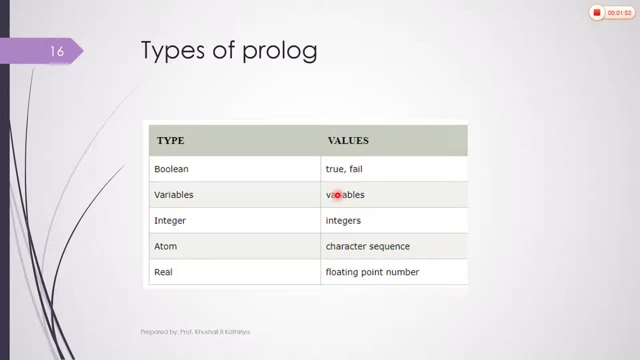 That means integer type means that you have a value that will be constant. That means there will be a number between 0 to 9. That's called an integer Atom. that means character sequence. Okay, you can say atom that means constant type. And what can you say to that Constant and character sequence? 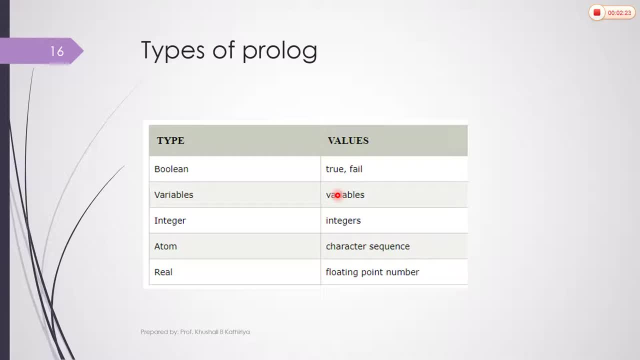 Okay, third one is the real. Real. that means floating point number. Floating point number, that means that you have an integer number. There is an integer number here, There is a character here, And what is the float number here? That means real number. Real, that means 1.2,, 1.3,, 1.4.. 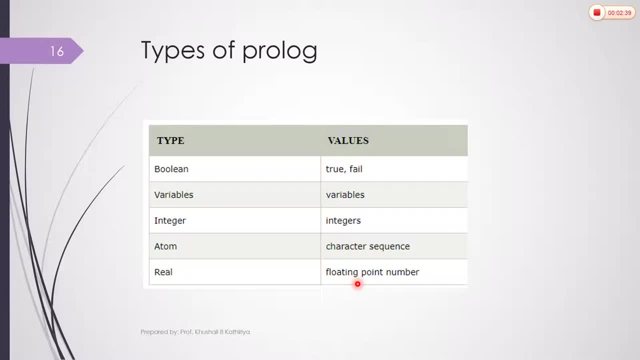 That's what happens. What do you call it? You can call it a floating number as a floating number. So in implementation, when we have to implement a prologue, then which types do we have? We will use the variables of the prologue. Or which types of functions, which types of predicates can we use? That means boolean variable, integer, atom and real. Okay, 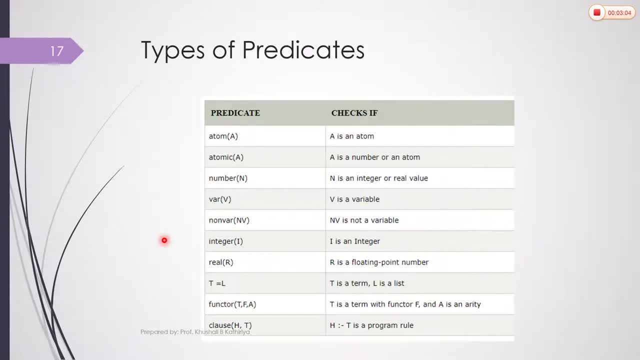 Second thing is type of predicate. Type of predicate: that means that you have, you have a parameter. What you have to do, What you have to do, You have to identify that parameter. That means its built-in function. What do you have to do with that predicate? By default, he By default. that means you have to do with him. 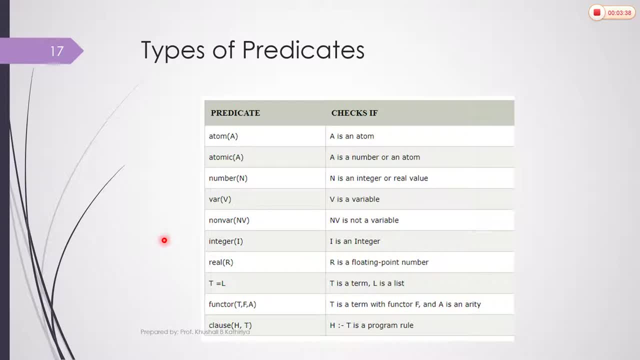 what to do. You have to consider it. You have to determine how he checks it in the prologue. So here the predicate and checked in. Okay, What does that mean? I have been shown that atom That means is an atom. 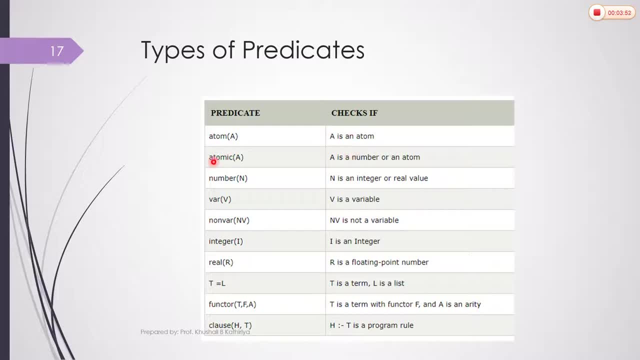 A is an atom. A is an atom. atom guy is a atom. okay, atomic, a number or a n atomic who character be was there, or number be was that number and that means it may be a integer value or real. will you okay where that means variable, non where that. 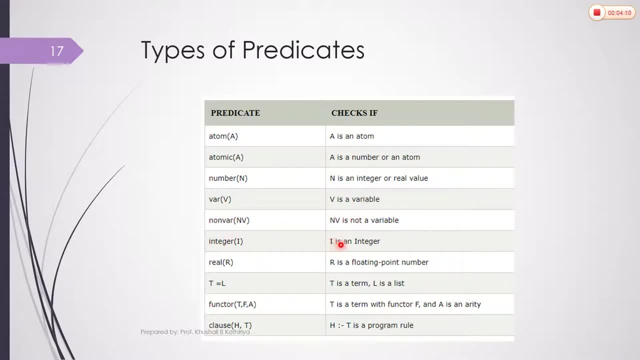 means non variable integer, that means the compulsory integer. okay, yeah, per number head, though maybe integer or real. that means 1, 2, 3, 4, any kind of or real number. one, point two, one point two, middle point, Wally Joe value with a woman. but yeah, per integer, head of pure integer over here, but real head to pure. 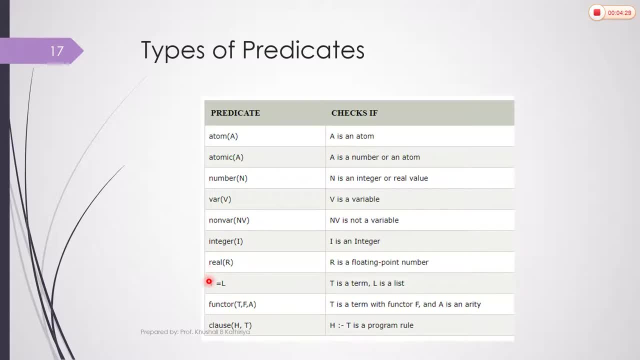 real floating number: Hoga, okay, I'll use as a list and TL use as a terms: okay, function, okay. us me a poor functioner made tf and a dumps us kajo go. every functioner have oh and last me every day. okay and clues love edge. 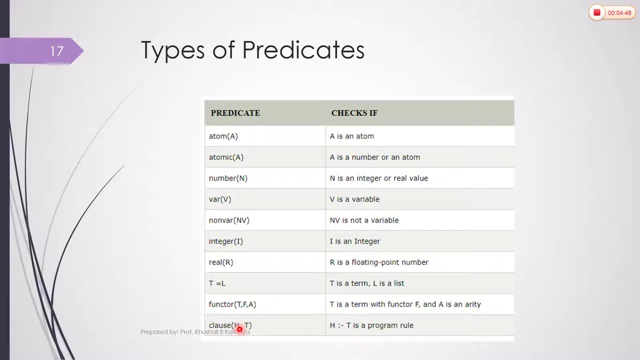 commodity with love. joke way, we have a a I'm gonna have to prove. Karna implies team and up to use a program rule. okay, I've got you a condition, it to you I'll execute. to be you. Allah clues obviously. fact we both up to okay, or is it you both up to term and list? don't know same. 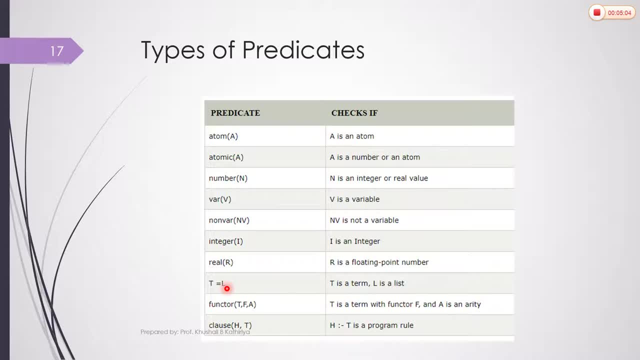 as a most of the other app, who is, in terms of X and Y, don't know where, variable, a local abuse turner and or up to bar bad measure of a person who's equal a number, then I have to feel the same. consider, can I? then you can use T. 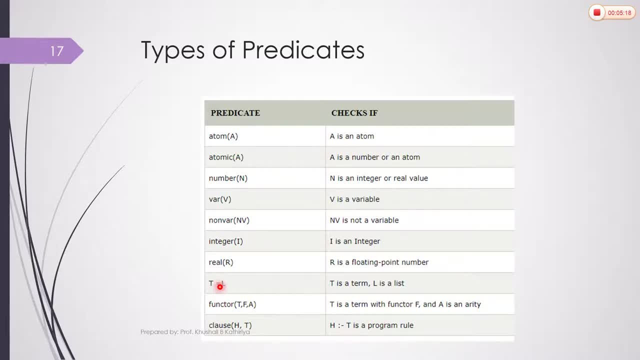 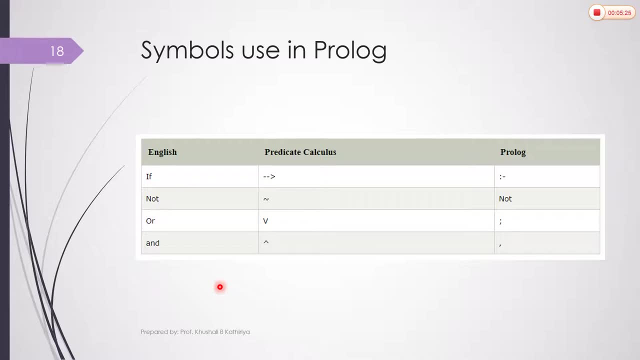 is equal to F, or we can say like that, X is equal to Y. okay, symbol use: which kind of the symbols are used? in a prologue, that means they are used, if not. or an end: okay, if we want to consider our knowledge made, knowledge based representation, that means we have 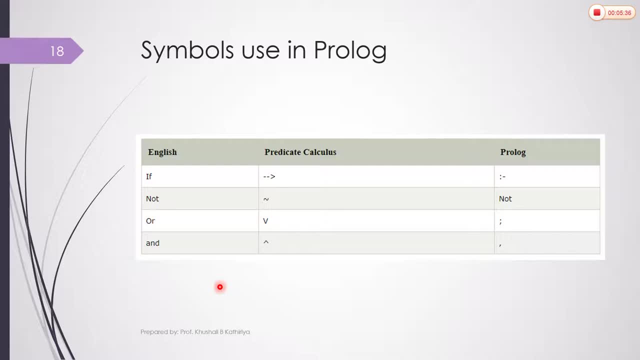 English sentence. then after that we have a convert into a predicate logic. but predicate logic cannot contain implies, implication. maybe it's contain implications, sign, double implication, sign and function or function not function. then if we use if function in our prologue, then what is the actual sign for the if? 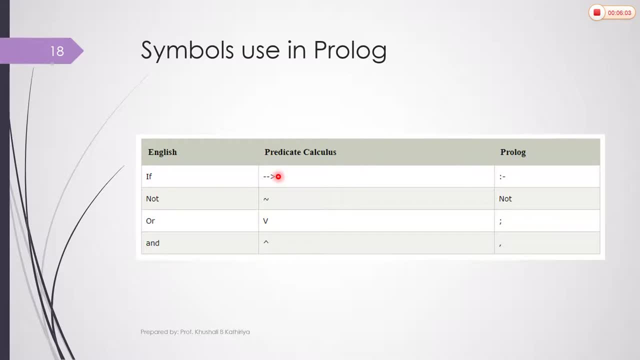 function. that is a implication, simple implication: sign dash, dash, greater than dash or greater than. but when we talk about the prologue, then we use the prologue sign as a colon dash. okay, we cannot use a dash greater than sign, but we have a used or colon semicolon, sorry, colon dash function after that. if we talk about the not 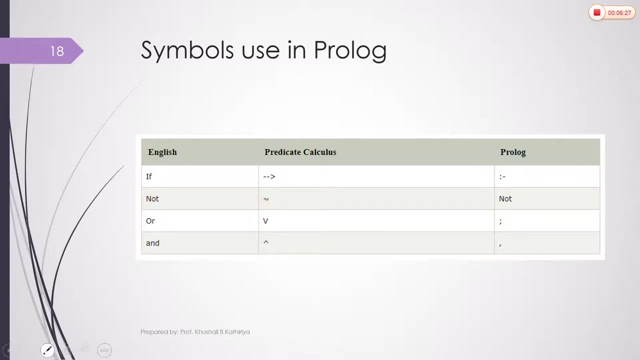 function not. that means not okay. we can also like that, write like that, okay, but the they are in our regular day-to-day life. if we talk about the not function in our books, and all okay, no function here or not. English to a sentence and no. but if we write a not function in a prologue language, then we directly use as a not. we cannot. 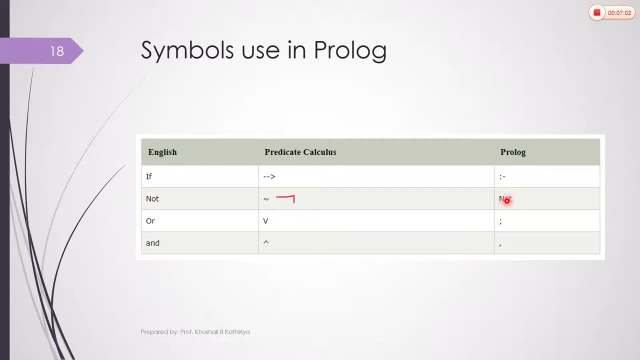 not use a sign, any kind of sign for the not okay or function- simply they are or. and end function- simply they are or and but or function. prologue used as a semicolon and function sorry. and function used as a comma. so in a prologue function we used if as a colon dash. 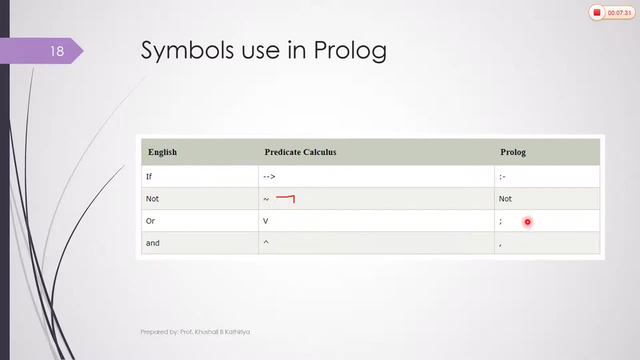 function not as a not or function: use a semicolon and end function: use a colon. okay, so this one is the symbol used. which kind of the symbol used in prologue? these kind of the symbols are used for the english sentence like if not, or and end. okay, 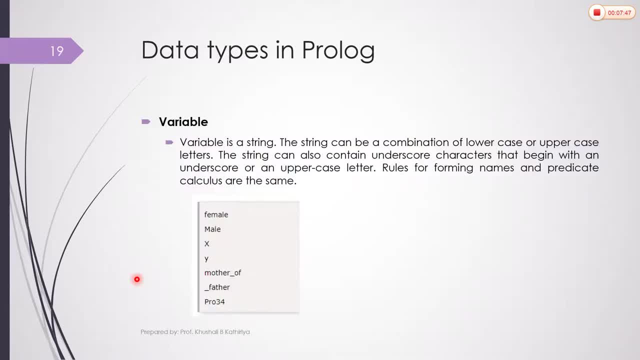 another is the data type. which kind of the data types we will used in prologue? okay, normally, but if we talk about the few, few data, by how few data types in a prologue, then first one is the variable: how to declare a variable and how to use the variable in a prologue. then where variable? 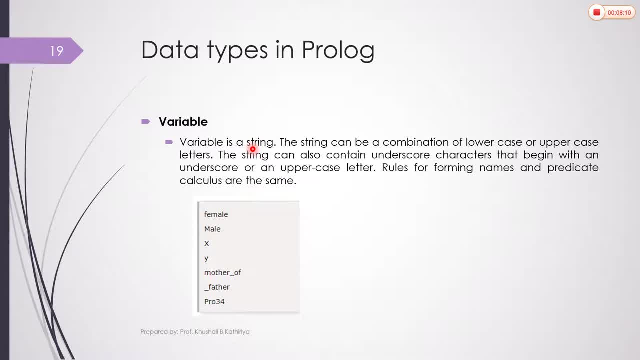 is a string version. okay, variable, kya hoga string. maybe it's a character, maybe it's a string, okay, so variable is a string. the string can be combination of lower or uppercase letters. the string can also contain a underscore character. that, beginning with, begin with a underscore or an upper character. 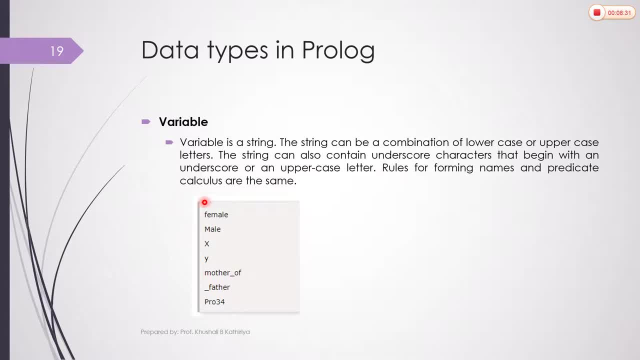 letters. okay, rules for formatting names and predicate calculates are the same. maybe our variable can be a character or a string. if it is a character, then it can be in uppercase and lowercase. this one is uppercase and lowercase, both our variable, its first character is capital and second last. 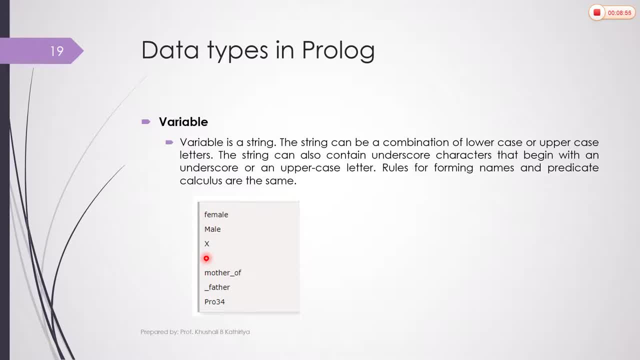 other remaining characters. it may be used as a lower character. we used a underscore function in beginning of our variable name and we we have also used, or we should also use, the underscore function middle of our variable name. we can use a number as well as as a variable name. 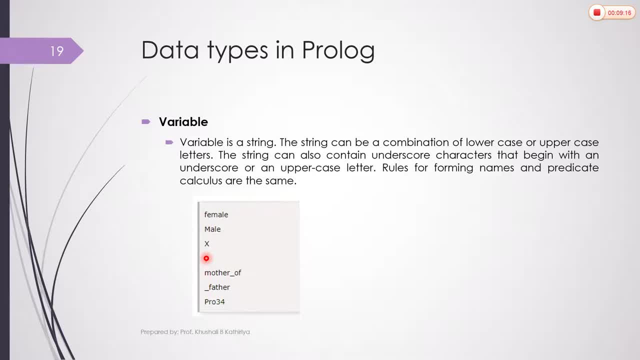 but number is not contain. our variable is not contain only numbers. they are contain number plus character. that means our number can't be a single number variable. that means you have to write some variable names, ie characters or a string in front. so this one is the. 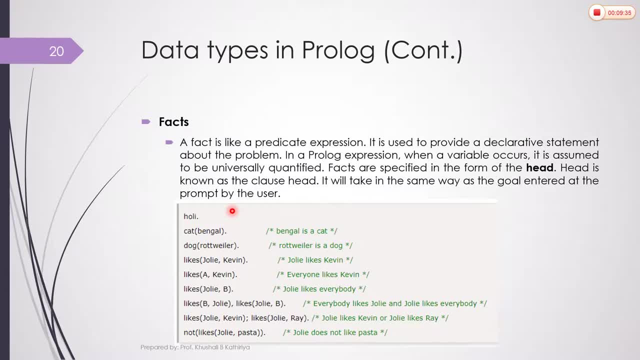 first: data: type of variable: how to declare a variable. after that we discuss a fact. fact that means what you have to do. fact is like the predicate expression. it is used to provide a declarative statement about the problems in a prologue expression when a variable occurs. 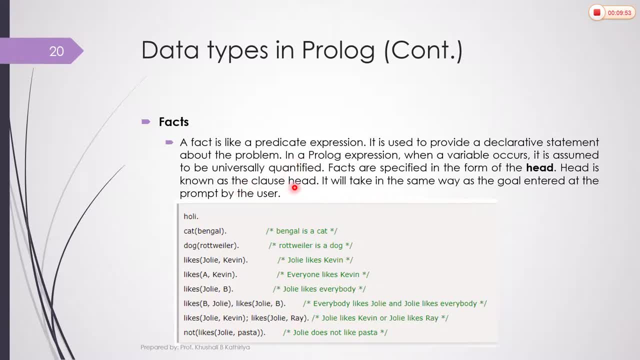 it is assumed to be universally quantifier. facts are specified in a form of the head. head is known as the clues head. it will take a same way as goal entered at the prompt by the user. here, what you have to do? fact, that means your predicate, your sentence. 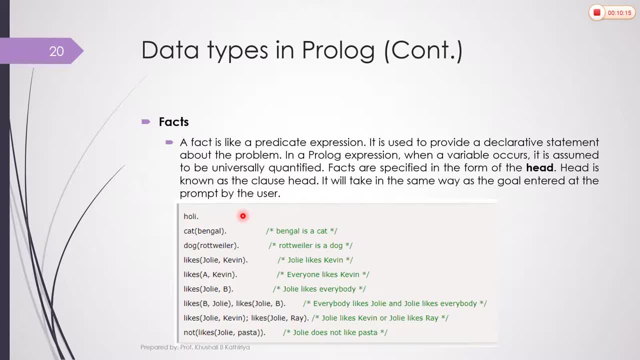 your English sentence. what you have to do with English sentence, you have to convert it into predicate. may be our English sentence, convert into FOL language and FOL language contain: and or if this kind of, not this kind of notation in our, in our, in our sentence. 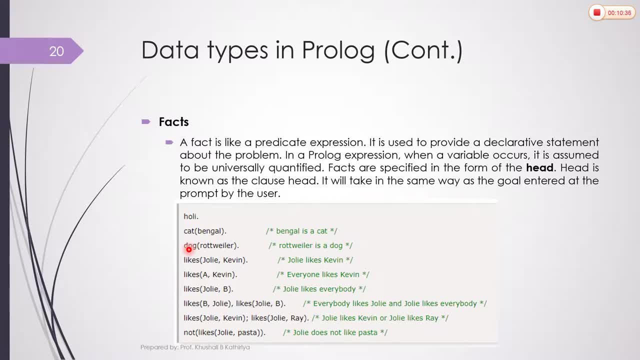 but we can use like that, we can use this kind of the symbols in our facts. so here these are the some example. like the bangle is a cat, then we can generate a cat as a predicate and bangle as a variable, ok, or name. so here we can use that. 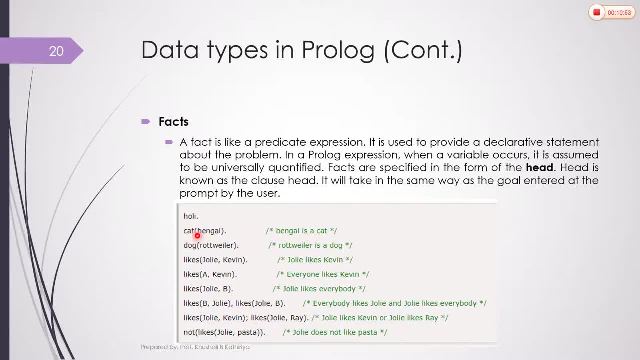 bangle is a cat, then we can say: cat in bracket bangle. ok. Rottweiler is a dog, ok, Rottweiler is a name of dog. then dog in bracket Rottweiler. jolly like Kevin. ok, jolly likes Kevin, so likes is our predicate. 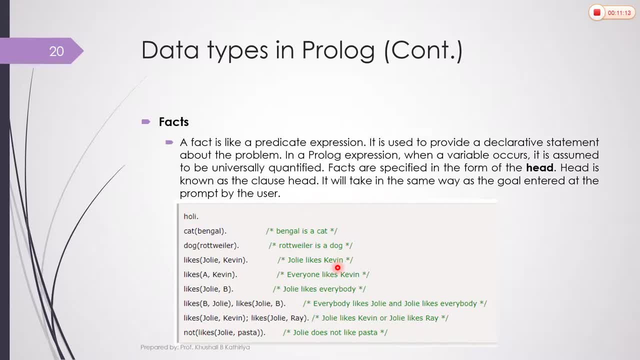 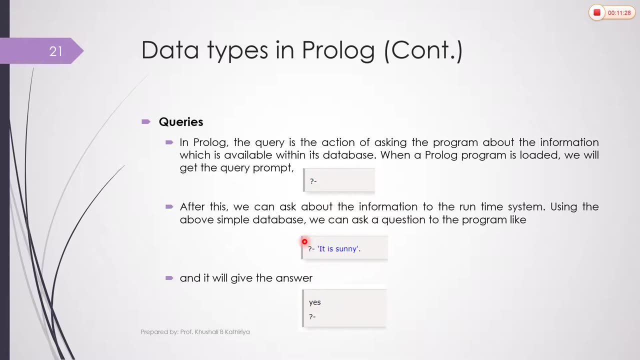 and jolly comma, Kevin, is our argument. ok. so this one is the simplest example for the fact. that means fact is nothing, but it is a conversion of English sentence to a FOL function, ok. another one is the query. ok, how to write a query in a prologue. 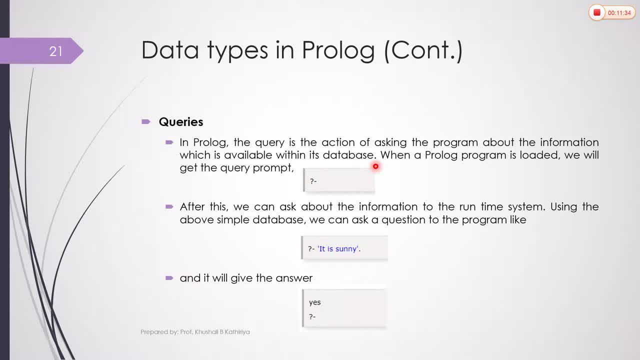 the query is the action of asking the program about the information which available, which is a database, when a program is loaded. so if we open our prologue screen or SWI prologue screen, then we see this sign at our starting point. ok, that means a query. 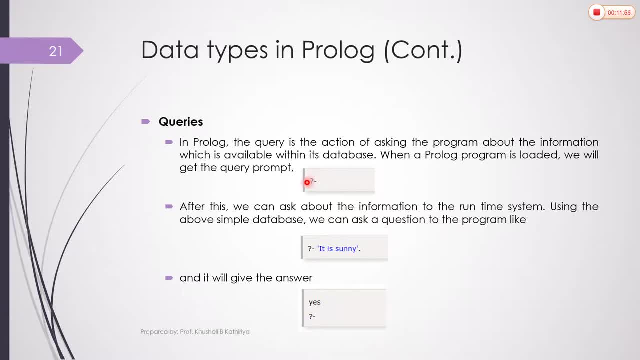 we can write here. we can write here as a query. after this line, we can ask about the information to the run system. using the above simple database. we can ask a question to the program like this: is it sunny? ok, is it sunny if this sentence is true. 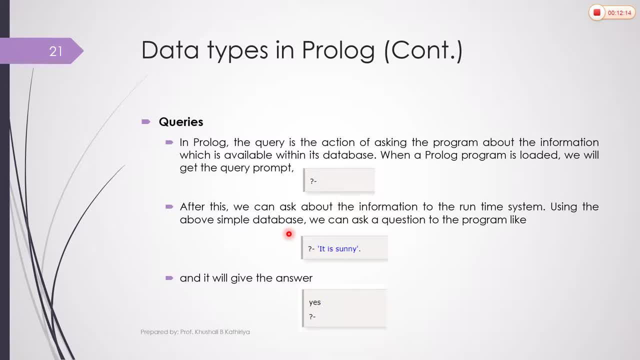 then what will it do? it will give a true answer. if that sentence is wrong, then what will it do? it will give a wrong answer. that means our sentence, our query, its answer: either it is true or it is false, like this, based on our database or based on our PL file. 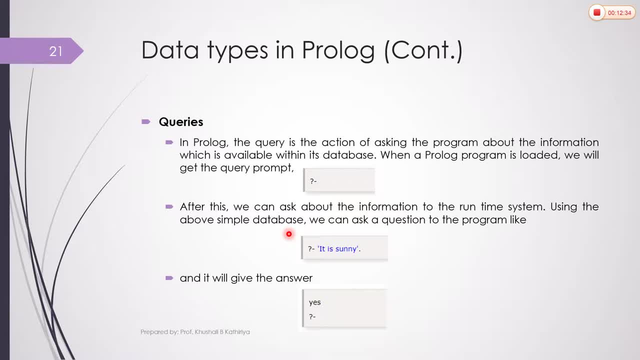 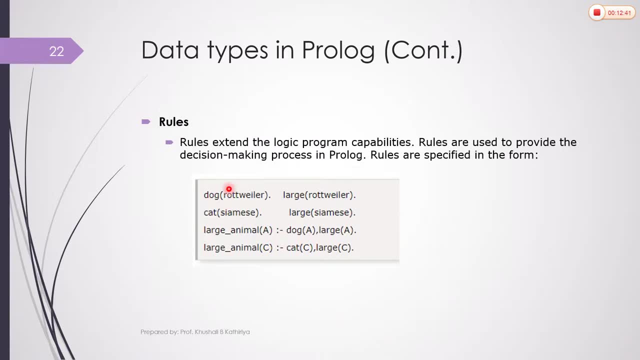 the PL file which we have compiled. based on that, based on knowledge base, our query will give us the output. another one is the rules. rule is extend the logic program capabilities. rules are used to provide the decision making process. in a prologue. rules are specified in the form: 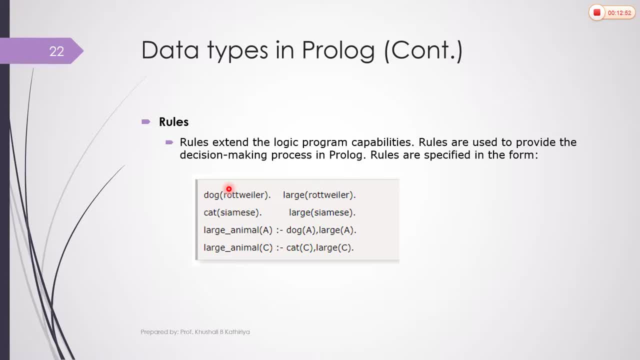 if we want to, if we want to understanding or if we want to generate a machine like a human commons file, then we can, we should provide or we have a. definitely we will get definitely good result during the if we want to generate any machine or any robotic machine. 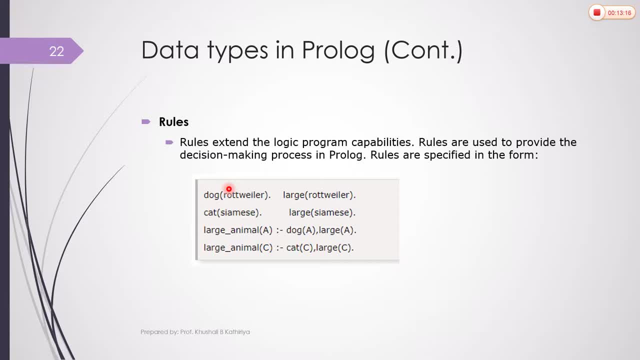 ok, then we must be provide a rules regulation to the machine. ok, if I give you an example here as a chinese room argument, which was our first chapter, introduction of AI. there we learnt Chinese room argument. what was in chinese room argument? what a person had to do. 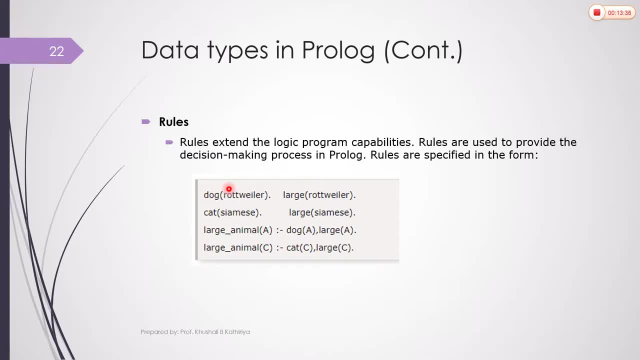 what he had to do he had to do in chinese, he had to give output, but he did not know chinese. he didn't know chinese language. so what he used to do- he had a dictionary in his dictionary. what he used to do in his dictionary english to chinese was converted. 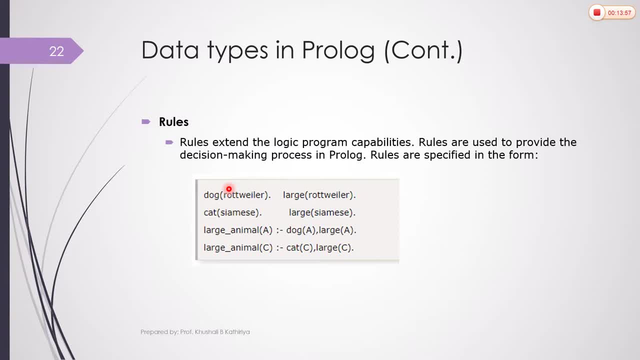 whenever he got input- meaning he got query- what he used to do, he used to find that chinese word in that dictionary. after finding that chinese word, what he used to do, he used to translate his english. after translating his english. what he used to do, he used to answer. 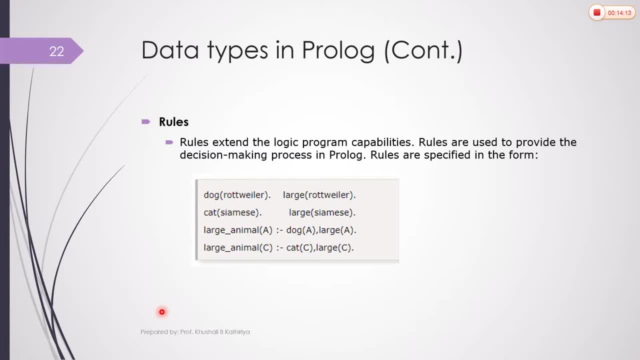 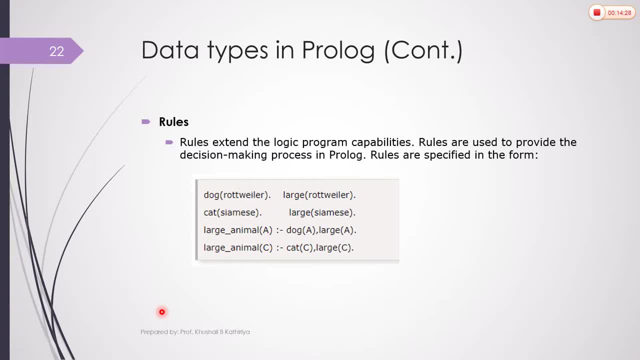 it will convert from English to Chinese. that means what was its input? input was Chinese, but what rules it was using? how to convert a Chinese language to English? after that, they use English to Chinese and they give output as a Chinese language. so what were those rules for that person? 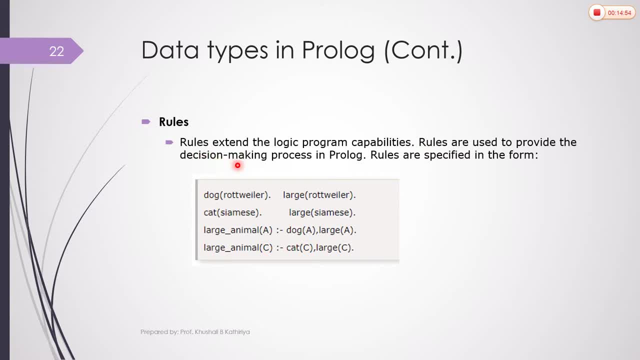 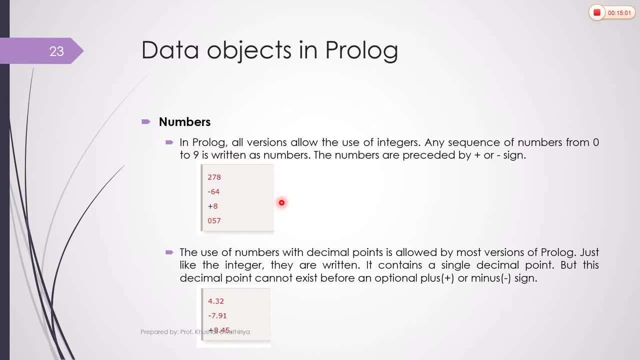 for that machine, then this one is your rules for the prolog. another data object in a prolog. that means a number in a prolog. all version allows the user of numbers. any sequence of number from 0 to 9 is written as a number. it may be use a plus and minus sign. 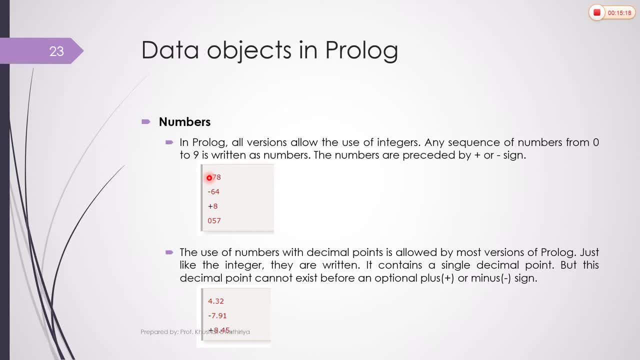 it may be plus or minus sign, any kind of like that. this one is example for the number. another is the real number if we used single decimal point, if we talk about the real number, if we talk about the floating number, then this one is the example for the decision number. 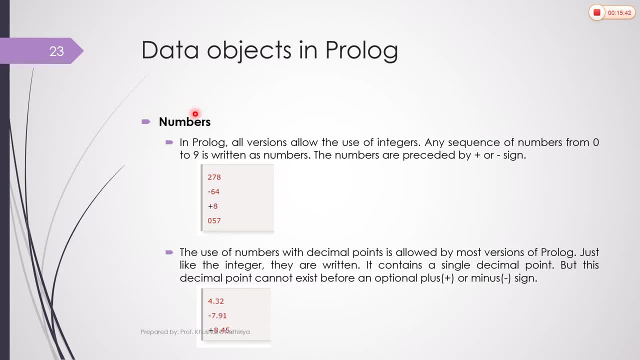 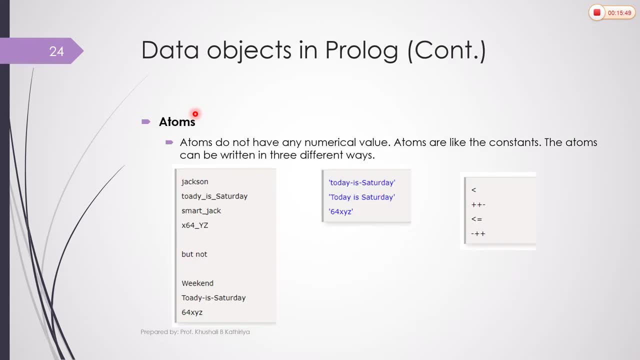 but number, contain both integer value or real value. both, but integer value only contain integer numbers. sorry, integer value and real number only contain real numbers. ok. next one is the atoms. atom means atoms do not have any numerical value. atoms are like the constants. ok, they are the constant value. 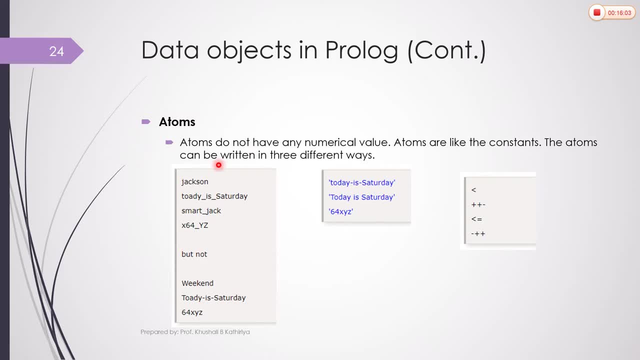 the atom can be written in any three different way: it may be totally character, it may be contain a string, or it may be operator or symbols. ok, here we have a string, sorry. we have a character, ok, we have a string, and this one is our symbol. so atom may be numbers, may be string or may be character. 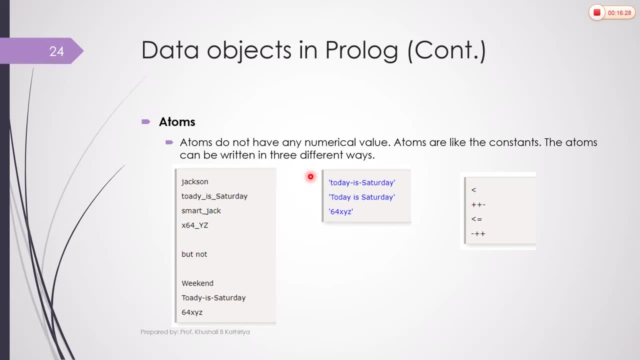 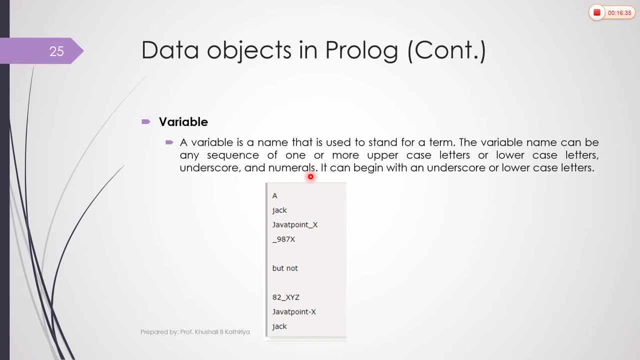 or may be single character, ok, so this one is always constant. another thing is a variable, ok, another we have already discussed in our data typing. first of all, variable may be contain a upper and lower case. it may be contain a starting middle, any, anywhere we used, we use underscore function, ok.